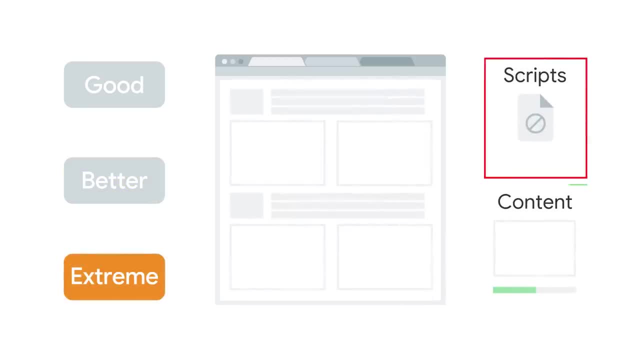 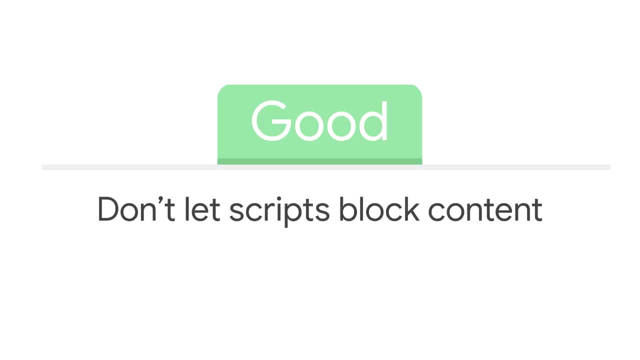 Extreme When you can make it so. most scripts don't even start to load until visible content is complete First. That's the first level of goodness. Don't let scripts block content. When the browser sees a script tag, normally it won't do anything else until it loads parses. 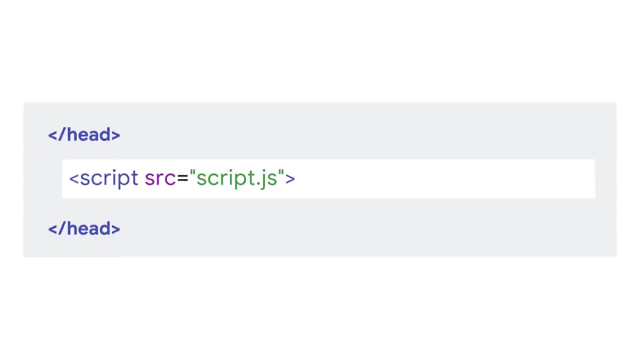 and executes that script When that script tag is in the head. this happens before it loads or shows anything in the body, In other words, before it shows any visible content. The process the browser uses to display visible content is called rendering. When a script blocks rendering, we say it's render blocking. 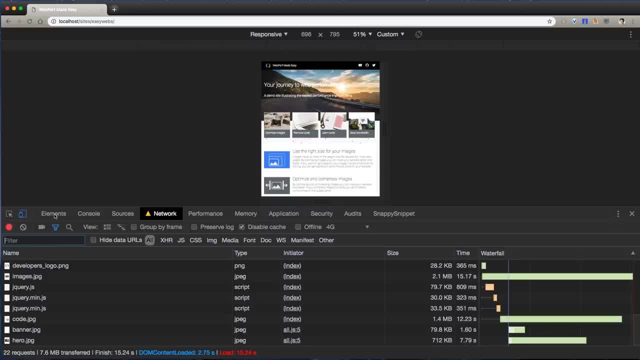 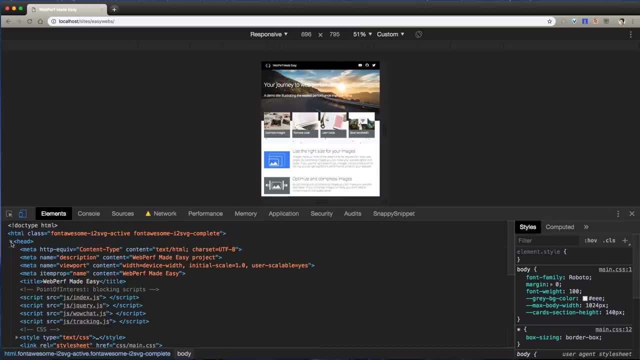 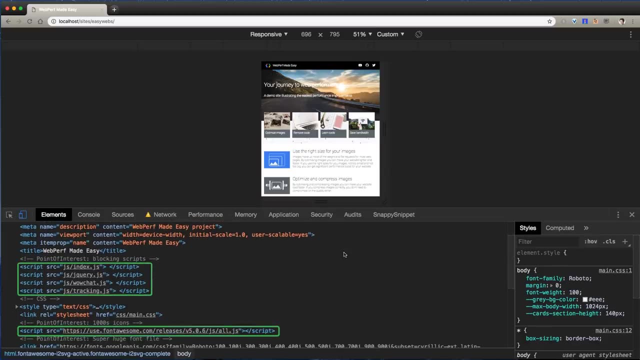 OK, Let's look for render blocking scripts in our site. We open up DevTools, then load up the site. We click on Elements. Right near the top is the head. We click on the head to expand it And look at that. we've got five scripts right in the head. 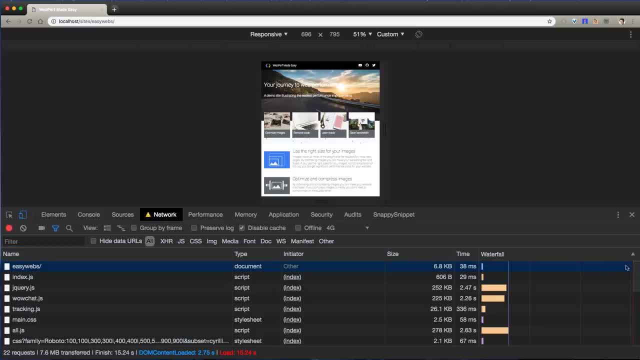 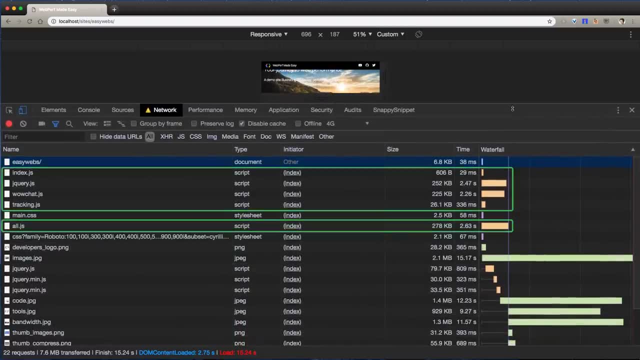 In the Network tab you can see that these scripts are render blocking. Look at those five orange bars in the waterfall. Those are scripts. Notice that they load fully before images even start to load. Now some scripts need to load in the head. 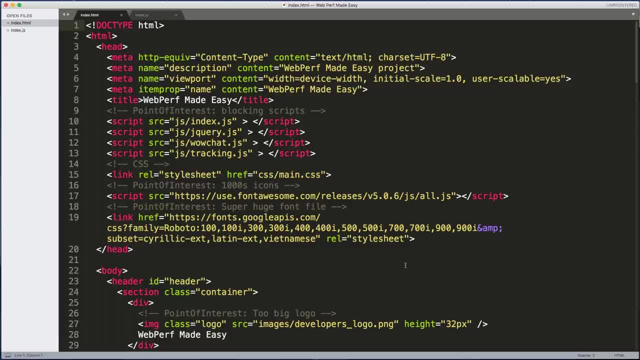 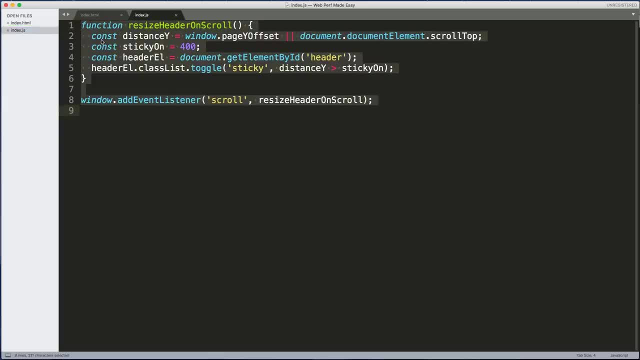 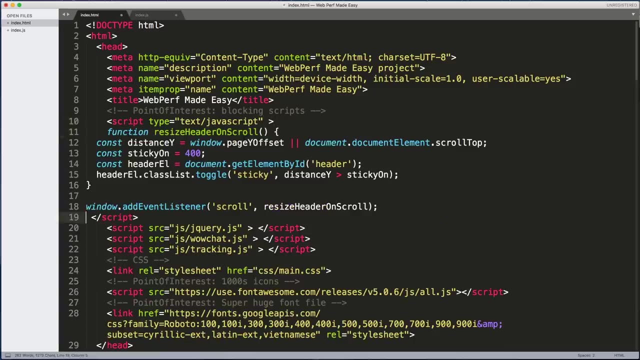 Sometimes jQuery does, but most scripts don't. Indexjs is really small and it looks to me like it should execute early, So let's copy its JavaScript right into the HTML. That saves a request. Let's leave jQuery where it is too, though it should be minified. 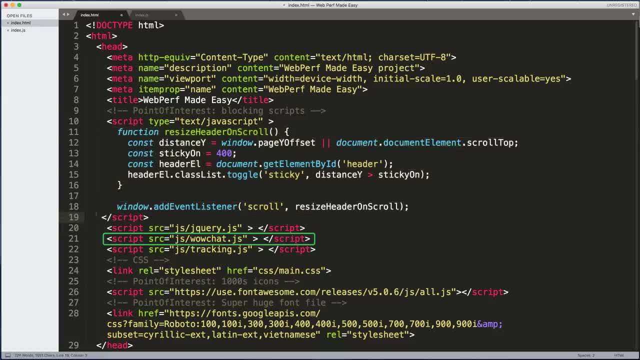 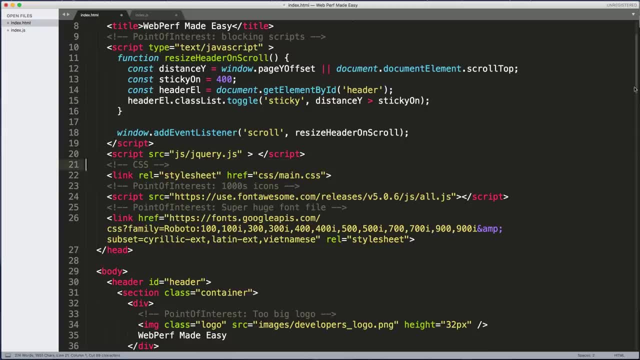 But do we really need to load that chat JavaScript before VisibleQuery? I don't think so. So next we'll take these other large scripts out of the head and put them in the body. Where should they go? Well, why not put them at the bottom? 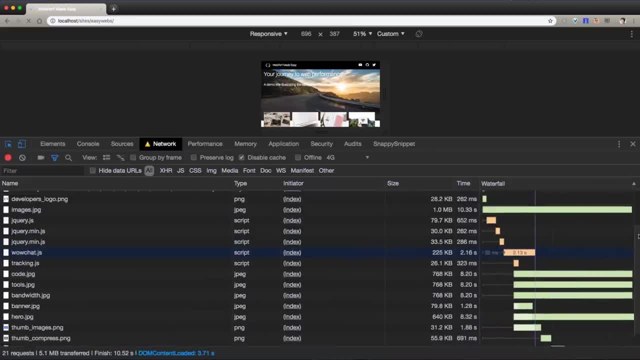 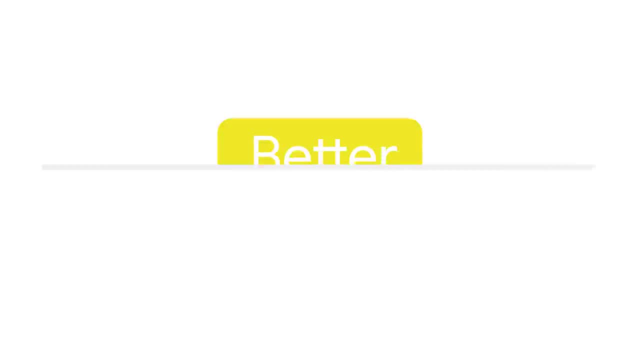 Wouldn't they load last? The bottom is good, But unfortunately, even if you put scripts at the bottom, browsers will tend to load them early anyway. So let's go to our second level of goodness, using the async and defer attributes. Async tells the browser that the script can be executed asynchronously.